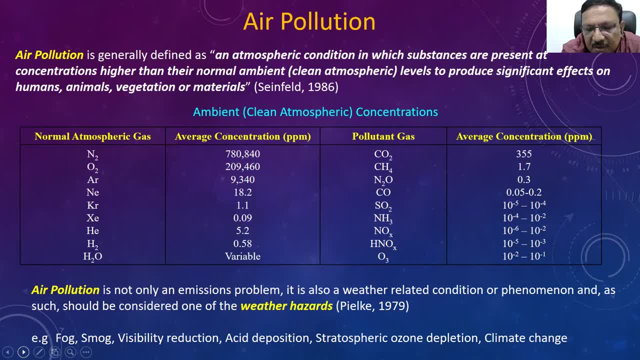 concentrations, the trace amounts of pollutant gas are there in the atmosphere and, as we know, air pollution is not only an emissions problem. it is also a weather-related condition or phenomena. as such, it should be considered as a weather hazard, like we have the smog and visibility. 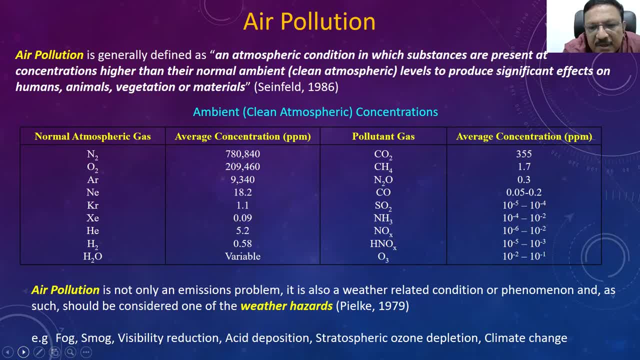 reduction, climate change problems, ocean depletion. all that and because of the emission of the air, pollutant gases and particulate matter in the atmosphere, in the foggy conditions in winter- the famous example of delhi and northern north indian cities- we have a lot of smog, because of which the visibility gets reduced and several flights get cancelled and trains get. 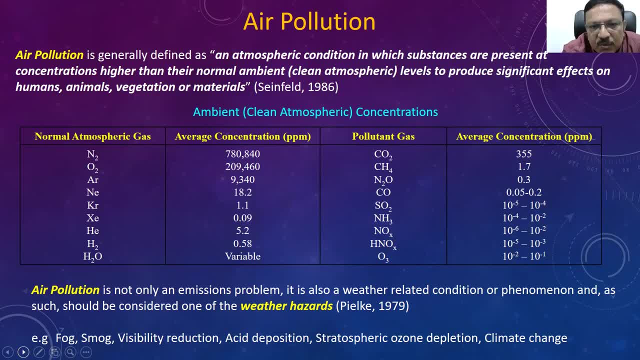 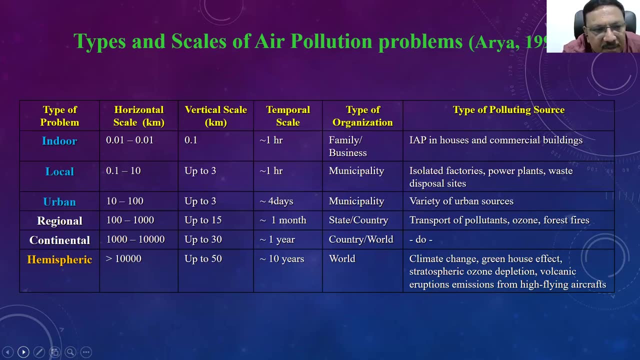 delayed or cancelled like that. so as such, the air pollution also should be considered as a weather hazard. next slide, please, and we would like to look at some of the types and scales of air pollution wherein we have, depending on the horizontal extent of the horizontal dimensions and vertical 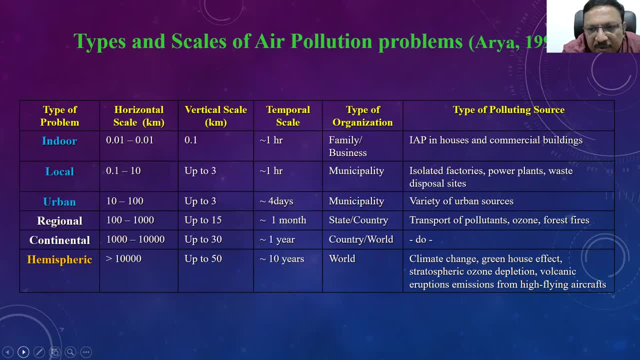 and on the temporal scale, what is the level of sources will be there in that area like and what are the associated sources will be there in those areas and types of air pollution and the broadly they can be put into three categories, like indoor, local types of air pollution, regional, continental, hemispheric and in the indoor, wherein the 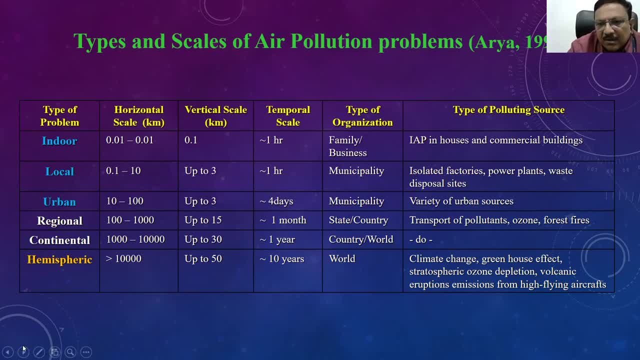 indoor air pollution in houses and commercial complexes or offices are where the human population will be there, which affected, which affects the people who live in that indoor regions. the horizontal scale will be up to 100 meters and vertical scale up to, say, 10 meters, maybe one. 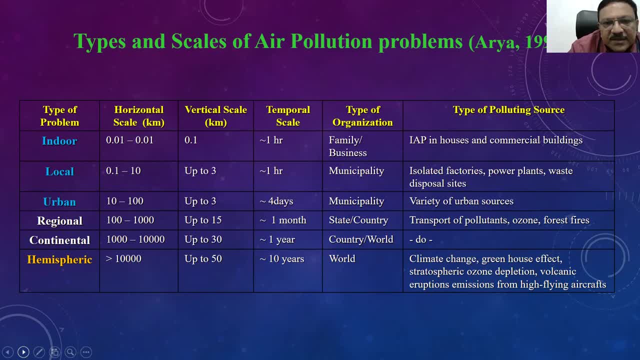 building height, a couple of buildings, two floor heights and up to the activity may be up to one hour, which impacts the uh human, uh humans dwelling in that indoor and, like museums wherein the artifacts were displayed, they also get affected because of the intrusion of the outdoor building. 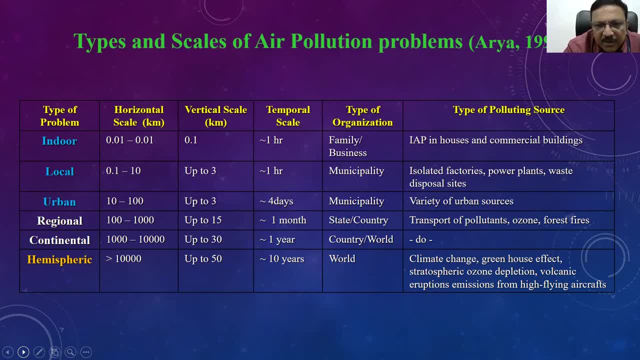 ambient air intrusion into the museums. that is called the indoor pollution. and in the outdoor pollution we have the local and urban which are up to, in the local areas, up to 10 kilometers extent in the horizontal and three kilometers up to height in the vertical, and the activity can be. 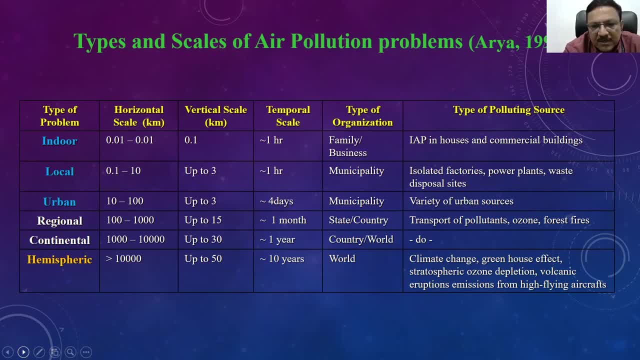 up to one hour, like the urban local bodies, like municipality or any ward of that municipality area, where in isolated factories or power plants or waste disposal sites or the vehicle movement will be there. all that will be taking place in that local scale. similarly, in the urban areas we go. 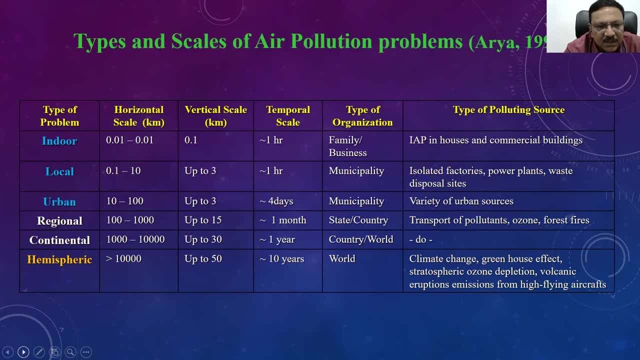 from 10 kilometers to up to 100 kilometers in the horizontal and up to three kilometers in the vertical, the pollutants can get transported and the temporal scale from hours to a few hours to up to four days, where, in a wide variety of urban sources, like, as i said before, the any formal industries or chemical 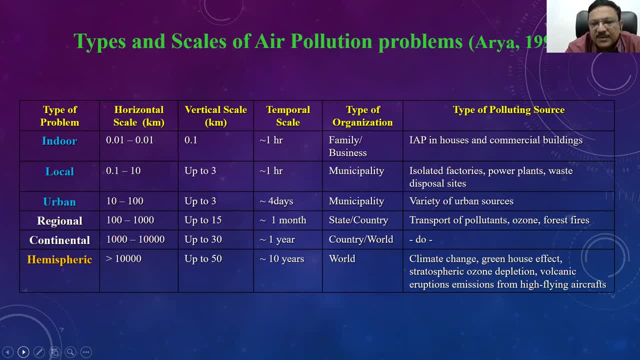 factories there in that area and the power plants in those areas and waste disposal sites, waste burning domestic waste burning solid waste transfering stations, landfill sites- all that along with the, of course, the major pollution from the regular sources. in any urban area or a city we have a lot many vehicles registered every day and there they have been playing on the. 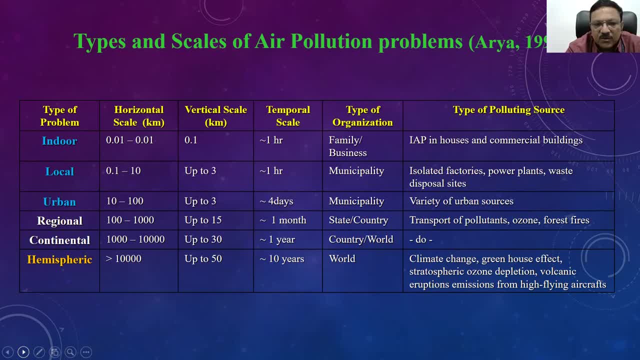 roads causing a lot of air pollution, and also the type of construction goes in the urban areas. the construction field also will add to the air pollution, along with the crematoria and other sources. and in the regional scale, uh, when you go in up to thousands of kilometers, you can see that. 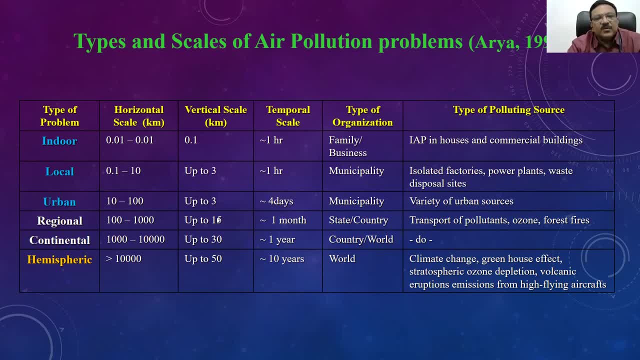 uh, here in the urban we have the business scale also. uh, we're in, uh, when we come to the discussion, we'll discuss that. and in the regional, up to thousands, uh thousands of kilometers and uh up to uh 15 kilometers vertical, like the beyond the tropospheric height, uh, the activities can be. 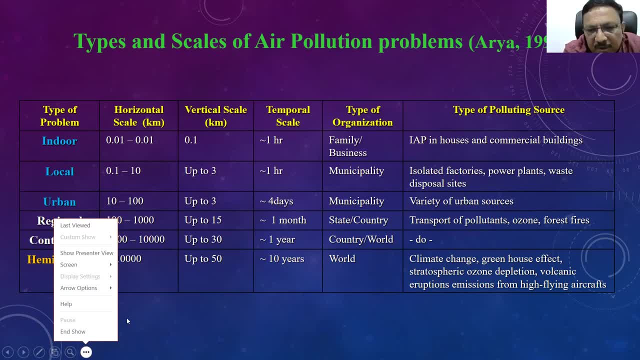 there up to a temporal scale of one month, from few days to one month, uh previously- and the the types of organization will be the state or country, the inter state transportation of pollutants, like in the case of delhi ncr, coming from adjacent states of rajasthan punjab, like that. 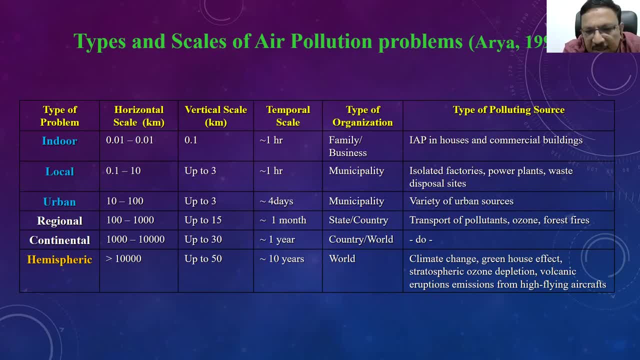 they are accounted for in this urban to regional scale. this is called the original scale of air pollution that is taken, taken by the transportation of pollutants and ozone. also in the vertical. uh, what with respect to the ozone? what we see is the stratosphere. the ozone formation will be there. 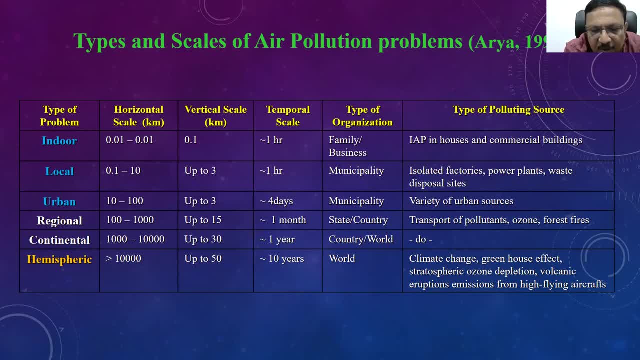 which protects the human beings from the ultraviolet radiation wherein the ozone will be treated as a pollutant in the troposphere and in the continental scale of pollution we have up to ten thousands of kilometers, up to 30 kilometers in the vertical, beyond the stratospheric lower. 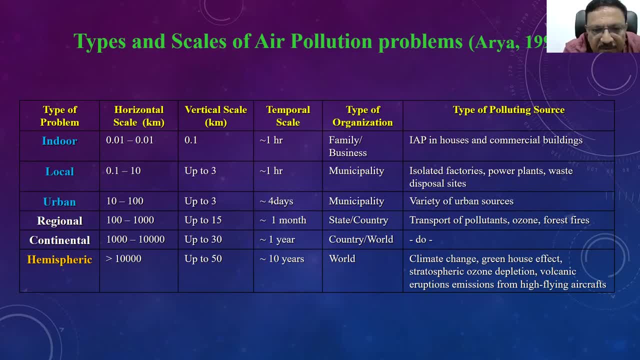 stratospheric heights up to one year of activities. uh, country and world will get affected here, in this case in the vertical, the in the regional and continental vertical scales, the chlorofluorocarbons and other things will get up to this. uh transported up to these heights and there has been in it, they'll be. 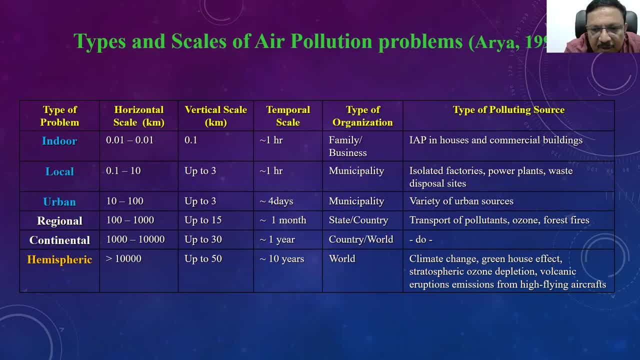 dwelling there for longer duration of time and uh depletes the ozone layer which we know very well. and the airplanes, jet planes moving across the world access the globe at those heights, also contribute to air pollution and hemispheric beyond the 10 000 kilometers up to 15 kilometers in the height and 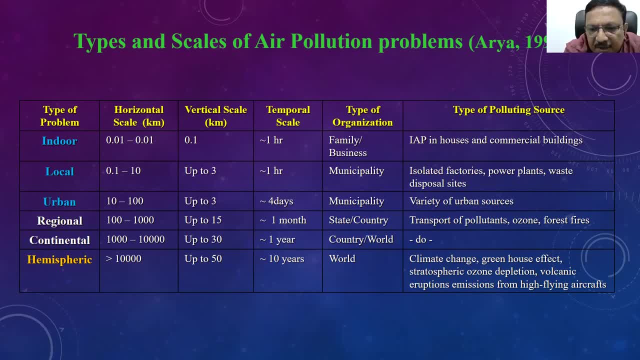 up to 10 years in worldwide where the climate change and greenhouse things are there. so, by knowing these types and the scales of air pollution issues, the kind of dispersion modeling or the kind of transport modeling, chemical modeling and other things like that are not going to be able to be used in this study, so i will leave it to you. 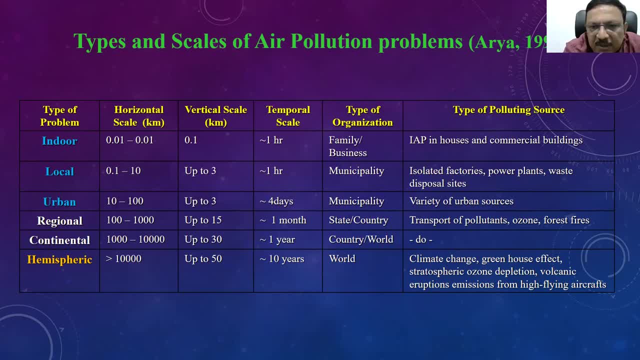 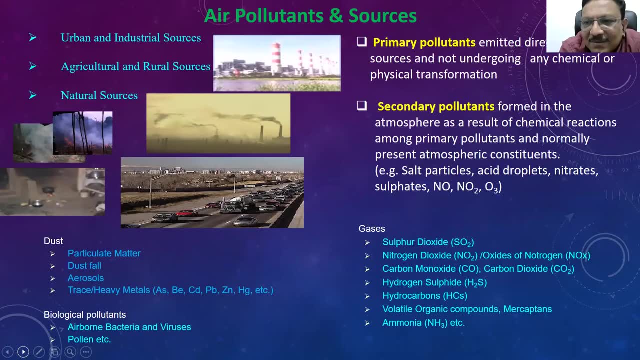 can be applied, which we'll see in the next discussion. Next slide, please. So, having known the definition of air pollution and the types and scales of air pollution, the air pollutants are primarily divided into two categories, like primary pollutants and secondary pollutants. 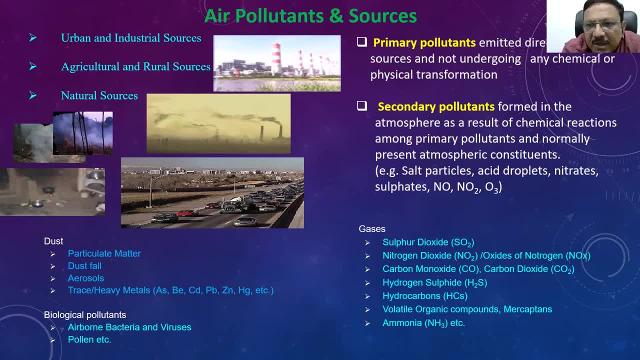 The primary pollutants emitted directly from the sources are not undergoing any chemical or physical transformation. They're called the primary pollutants And secondary pollutants, from which the primary pollutants released from the sources and when they enter the atmosphere as a result of feature, there will be reactions among the pollutants. 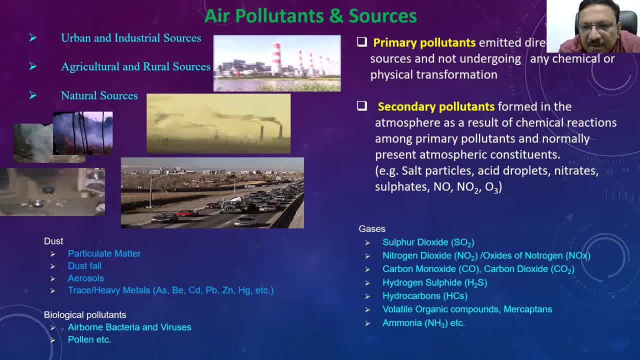 and the water vapor present in the atmosphere and associated pollutants gases, They'll get the generation of secondary pollutants in the air, like salt particles, acid droplets and sulfates and nitrates, because of which the acid deposition will be there. 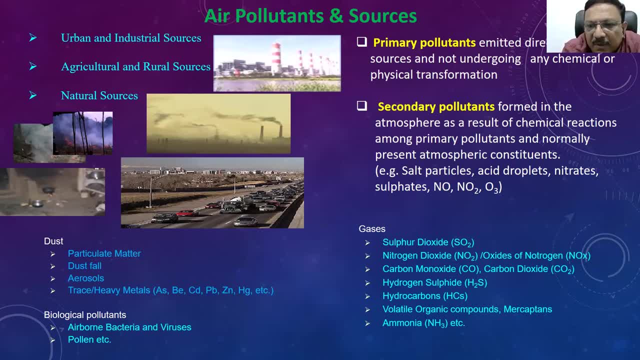 And, of course, ozone is another famous example of secondary air pollution creation And we have several sources, as we have seen in the urban areas. Industrial sources will be there. They're like power plants and the cement factories and all other small scale to medium scale industries. 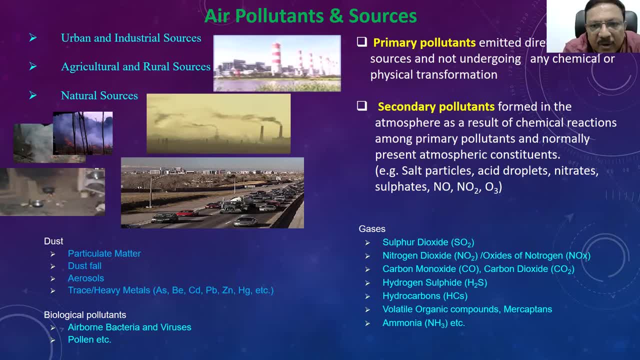 and different areas, et cetera. They all emit a particulate matter and that's what all knocks into the atmosphere. The agricultural, rural sources are there and the natural sources, like volcanoes and all, And in the urban sector we have the transportation. 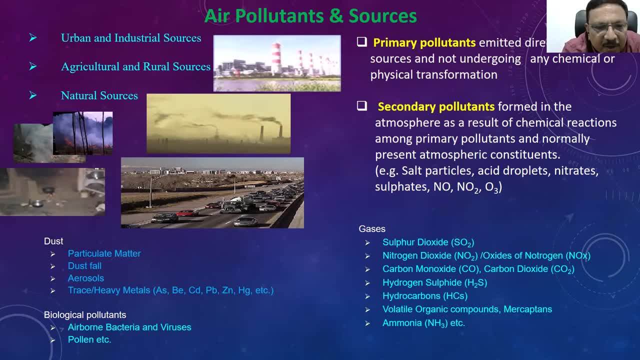 which is very highly polluting the atmosphere, the lower atmosphere, because of which a lot of health issues are also coming up, And knowing about these sources is important in the dispersion warning. And what are all? the main air pollutants in the atmosphere we encounter are the dust. 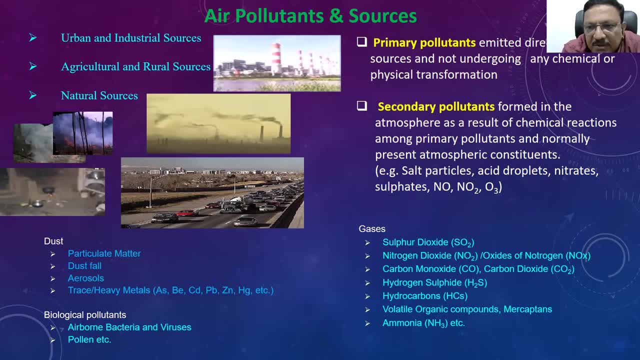 like particulate matter, The aerosols and particulate associated with the associated heavy metals like arsenic, lead, nickel, mercury, et cetera, And biological pollutants and gaseous pollutants like sulfur dioxide, nitrogen dioxide, and interaction with among the pollutant sources. 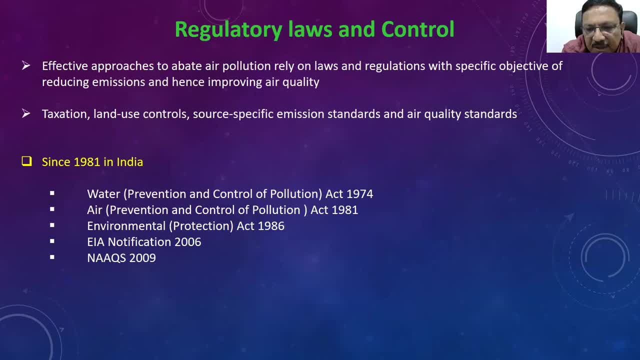 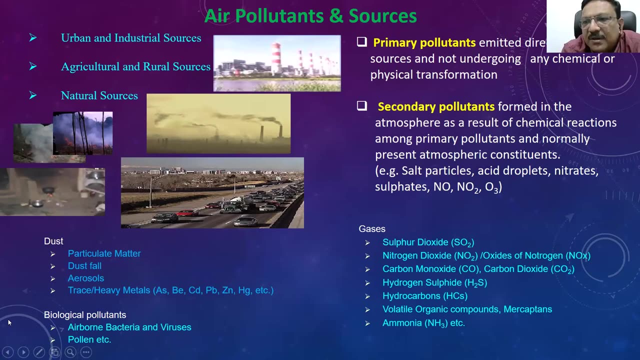 nitrogen also will be formed- carbon monoxide, carbon dioxide- which are already there- Hello, Can you? and the volatile organic compounds and the arduous pollutants like mercaptans, ammonia, et cetera, also will be released from different types of industries. 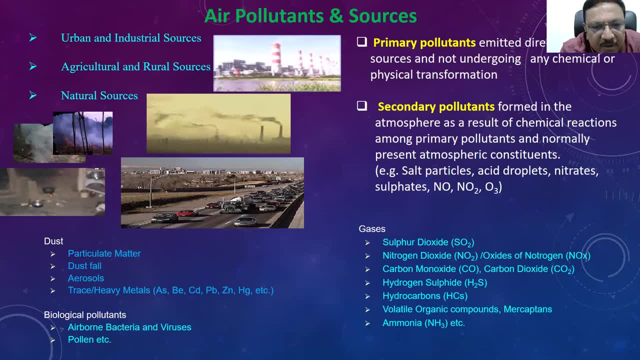 And we need to know about the. what are the significant pollutants and what are the significant sources in any urban area or any area wherein we need to treat them for studying the dispersion of air pollutants? The next slide, please. We all know the regulatory laws and control is required. 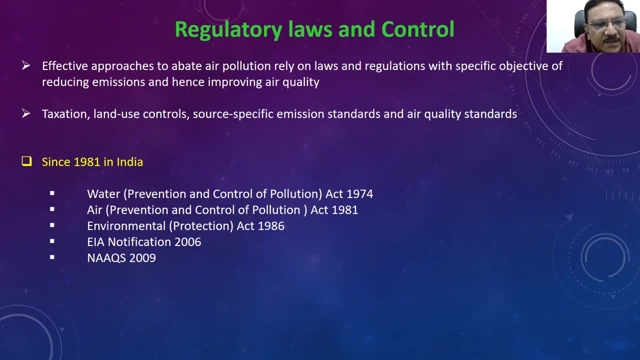 for effective approaches to avoid air pollution, wherein taxation, land use controls and resource specific emission standards and air quality standards need to be developed and reviewed periodically. There are laws in India since 1981, like Water Prevention and Control Act of Pollution in 1974,. 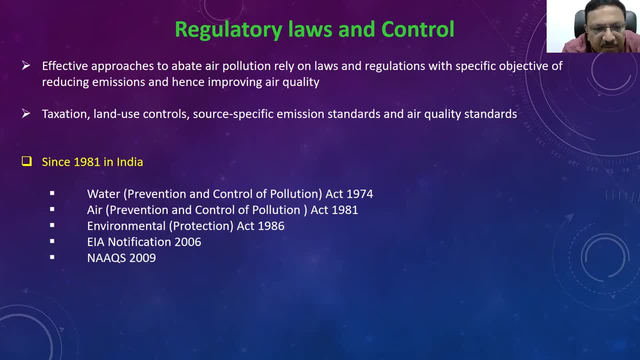 Air Prevention and Control Act in 1981.. Environmental Protection Act in 1986, after the famous Gopal gas tragedy. the EPA Act has come into picture and the AA notification has come into 2006 and is being reviewed now extensively, And the in the National Ambient Air Quality Standards. 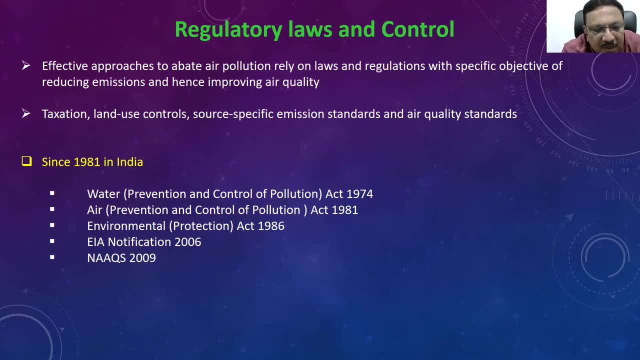 were prescribed in 2009,, wherein 12 parameters are given. Earlier we used to have only the classification. will be there separately for commercial areas. also individual areas, layer, but all these group together in only one category from 2006 to 9, and there are only two classifications. 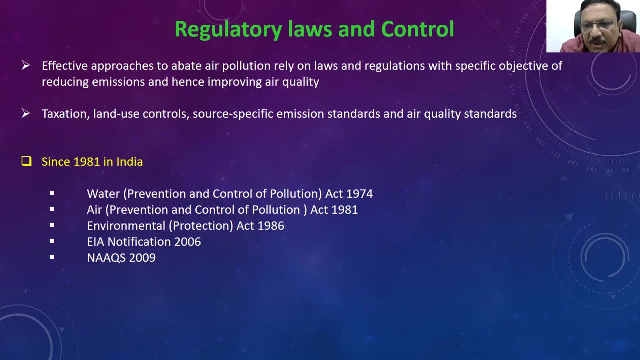 The industrial mixed use, commercial and residential areas are group into one And another for given standards for based on 24 hourly averages, and what is for auto layers, and also closing later And now having proportion on a maximum facade of India. BAP, the benzoalpha perine is also included. 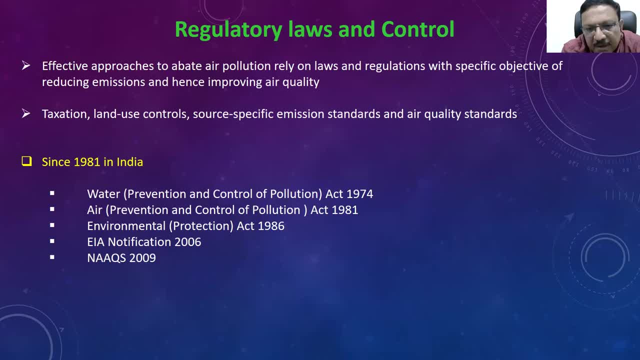 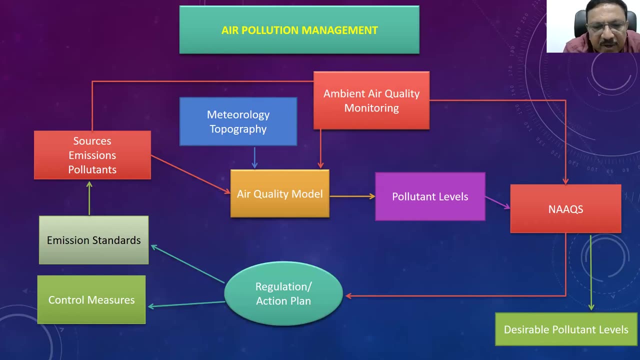 because it gives carcinogenic effects leading to the cancer. So several pollutants are included in the National Amphibious Air Quality Standards. Next slide, please. And for any urban areas or cities to have the city action plans are taking some regulations. The regulatory bodies have to be going through. 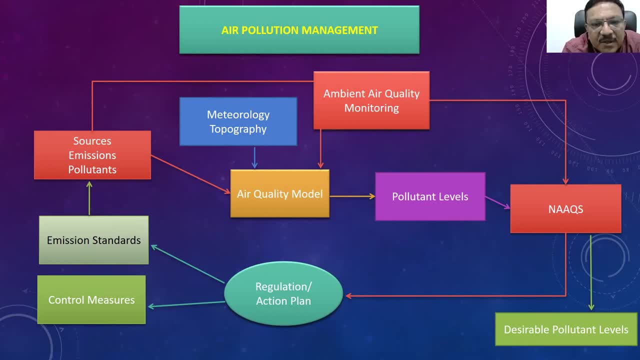 some air pollution management. The air pollution management as such will constitute the information on several things like what are the types of air polluting sources and what are the different emissions coming from that and which are the pollutants are specific in those areas, and local meteorology and local topography is required. 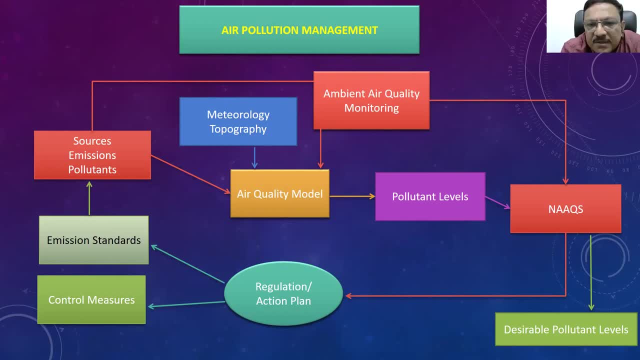 And the ambient air quality monitoring, which was extensively discussed by three parties here, where, in all the 12 kilometers and depending on the city, specific sources, the type of pollutants need to be monitored periodically and the database will be helpful for regulatory authorities to make the further improve. 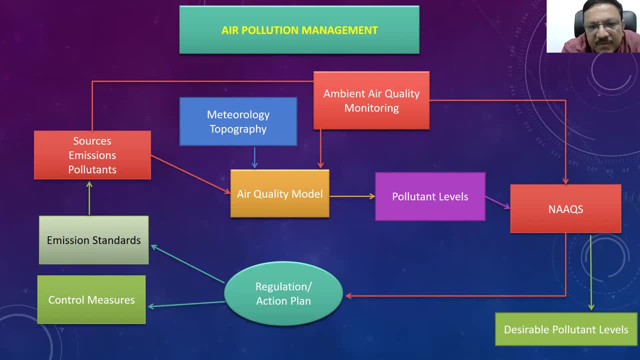 the National Amphibious Air Quality Standards or emission standards for which the air pollution model can be utilized. The air quality model is nothing but the dispersion model, the air pass dispersion model, which takes the inputs of the types of sources, emissions and various pollutants. 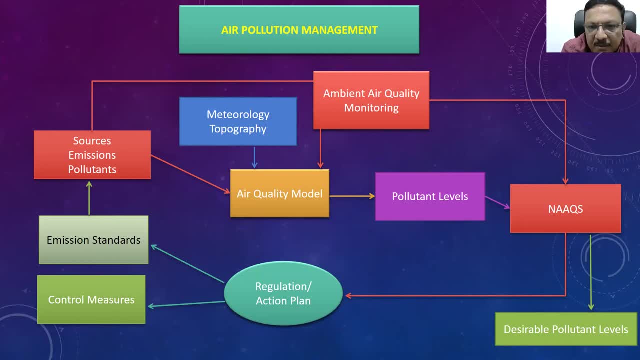 and local meteorology topography associated thing like any in the city, For example, any coastal area, is that coastal water is also considered in the study area And the ambient air quality monitoring will give you the background air quality levels. The model predicts the pollutant levels. 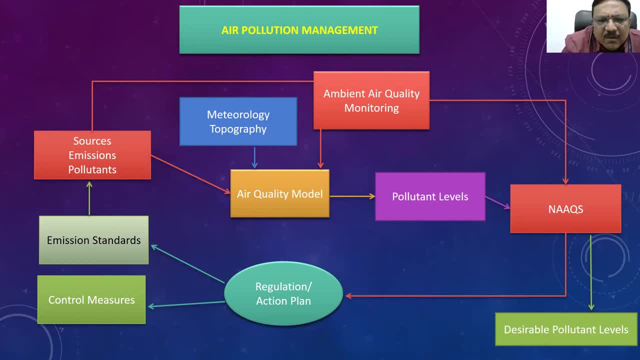 and with the monitored pollutant levels, the model predicted, the levels can be calibrated And again the desired pollutant levels can be opened by comparing with the National Air Quality Standards If they're far exceeding in any urban city. if the ambient levels of the pollutants are far exceeding. 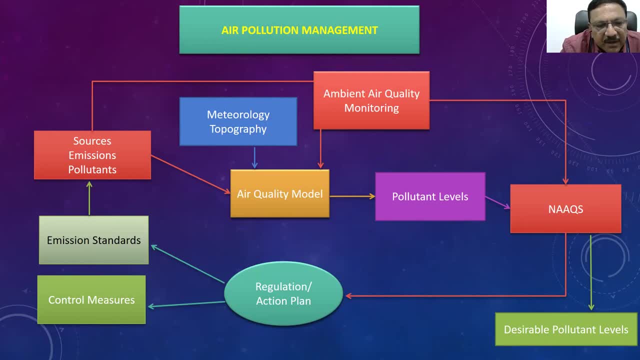 the standards, then there needs to be an action plan, a regulation, by using some control measures with the source and by putting the stringent emission standards for controlling the pollution from the sources, For example the emissions like from chemical plants, et cetera. 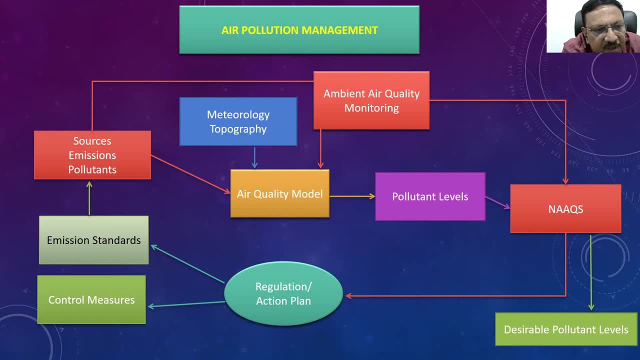 can be given stringent standards, For example the thermal power plants. the mercury emissions were given this time and the PM10 emission standards are also stringently reduced. So to take such kind of regulatory action, the atmospheric dispersion models or the air quality models will play an important role there. 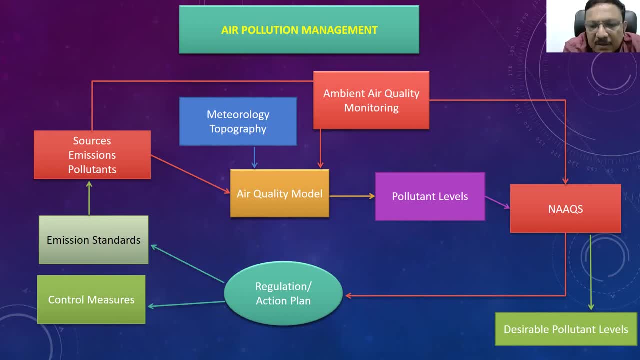 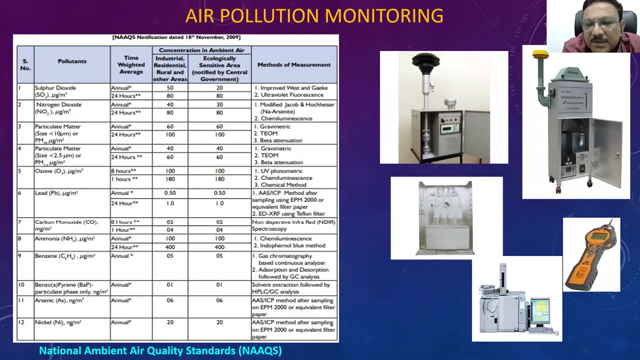 Which, wherein the district level planning or the urban local body level planning, will be made to reduce the pollution in those areas. Next slide, Next slide, please. And the air pollution monitoring which was already described earlier in extensive, wherein all the parameters need to be monitored. 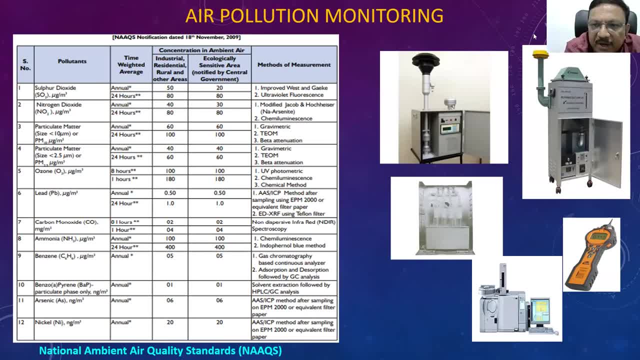 with our various methods And for the. as per the regulatory purposes, we use the RDA samplers and PM2.4 samplers and associated gases should be analyzed using the like, for example, SO2 modified as an example of a. 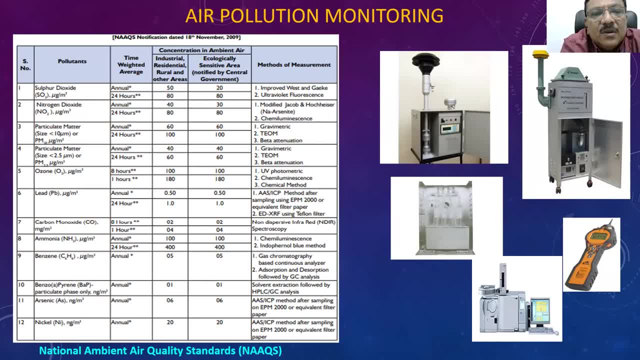 many may be about 15 to 20, or 23, or probably 15,. how many? not only 15,, but also speed. We use this in a couple of different ways, And the basic approach is that we will monitor. 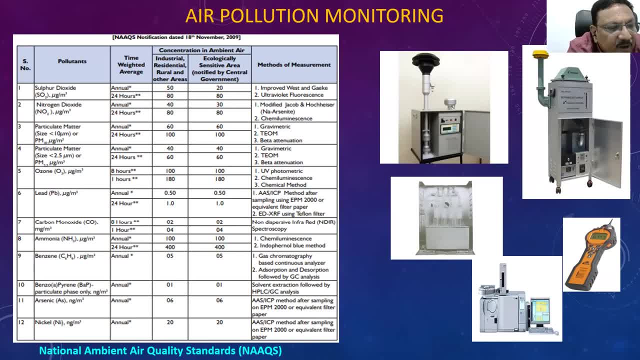 the. you know condition of the energy and the and the the industrial environment. And you know the. you know the environment can be courageously optimized and it's possible in the future. You know. you know we use� söz in the. you know in a as an example. 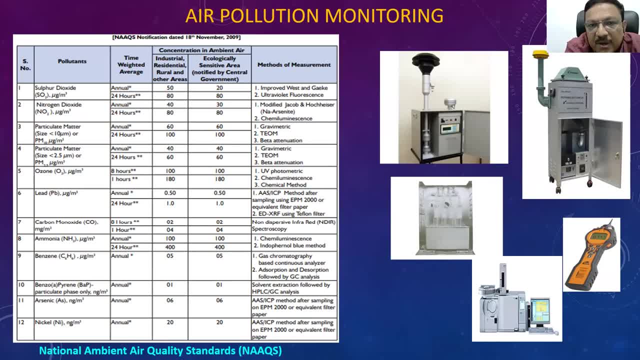 This monitoring is required to know the level of pollution in that urban area, which can be given as background information to the dispersion model, to estimate the pollution levels due to various sources in that urban area and then compare with these levels on national ambient air quality standards, the action plans can be prepared. 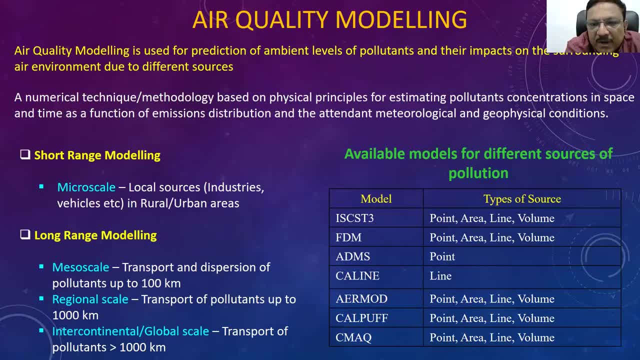 So the dispersion modeling will be another part wherein I would like to discuss about what is air quality modeling? It is used for the prediction of ambient levels of pollutants and their impacts on the surrounding air environment due to different sources: The different sources which we have seen previously, industrial sources and others, which is the 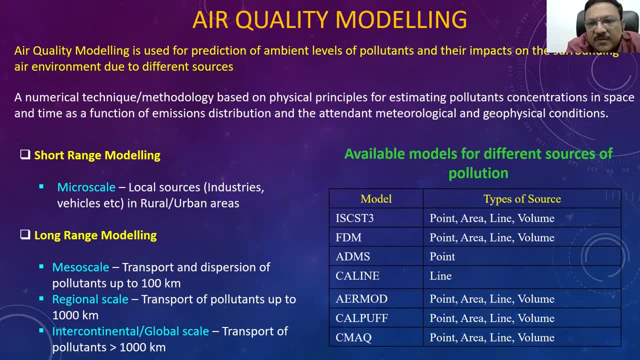 dispersion model is nothing but a numerical technique or methodology, Based on physical principles, of estimating pollutants concentrations as a function of time and function of emission distribution and the attendant meteorological and geographical features. Like you, need to give information on the local meteorology for knowing the dispersion turbulence. 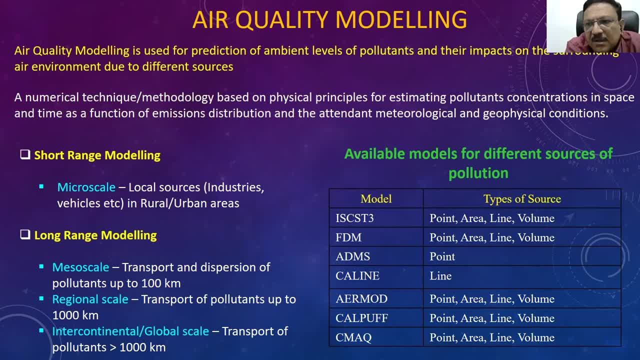 of the atmosphere and then the emission rates of the pollutants and characteristics of different sources need to be given. And again, the dispersion model. The dispersion model can be divided into two scales, like the short-range modeling and the long-range modeling, As when we discuss the types of scales, we have come across the urban and local sources. 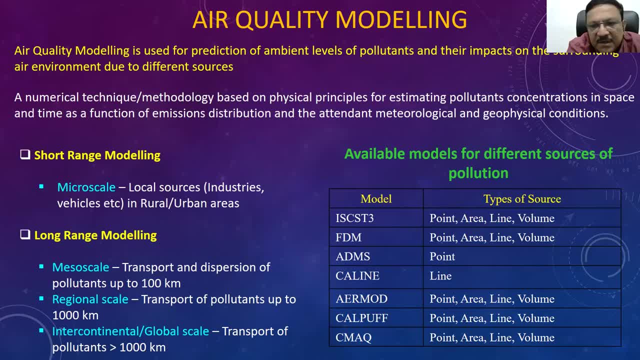 which comes under the microscale here. The local sources like industries, vectors, et cetera, and urban areas are treated with the short-range modeling And long-range modeling, the up to 100 kilometers, the transport and dispersion of the pollutants. 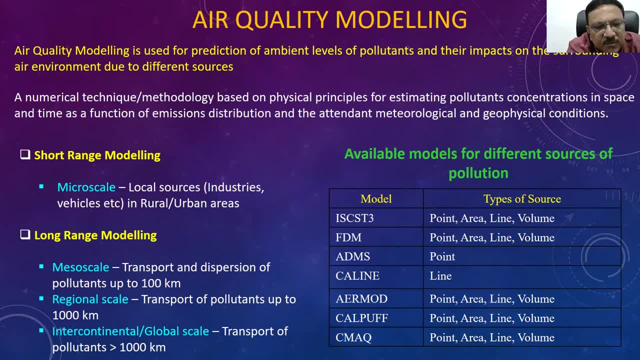 Up to 100 kilometers. If we take the dispersion of pollutants, We take it here at a scale transport of pollutants up to a thousand and intercontinental beyond the thousand kilometers, And in all these models one can have chemistry into it and we can know about the information. 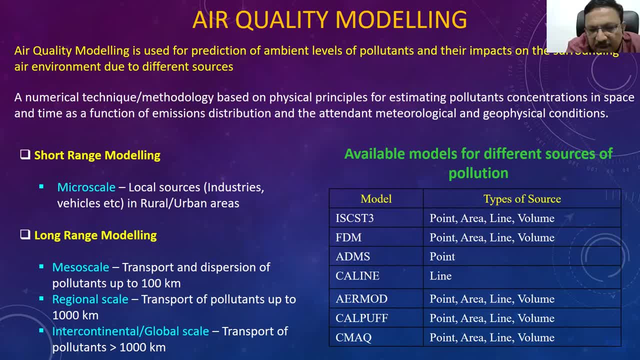 on the secondary pollutants- air pollutants also- But whereas for all practical purposes we'll be using the microscale in the urban, local and urban scale, wherein several models are available, Like IACs, The three industrial source complex short-term model and ADMS atmospheric dispersion modeling, 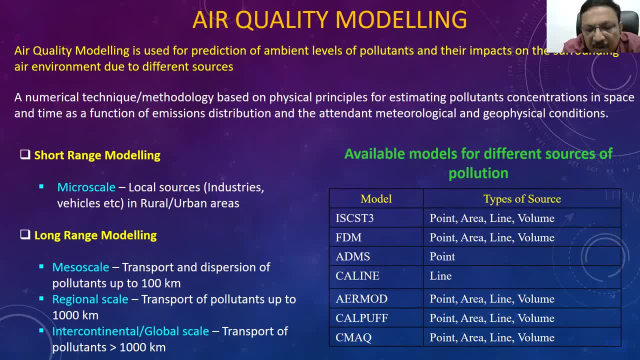 system, AERMOD, US EPA model, regulatory model and CALPF, CMAC, community multi-scale air quality model. like that, All these three models can treat the different types of sources like point sources: nothing but the stacks. 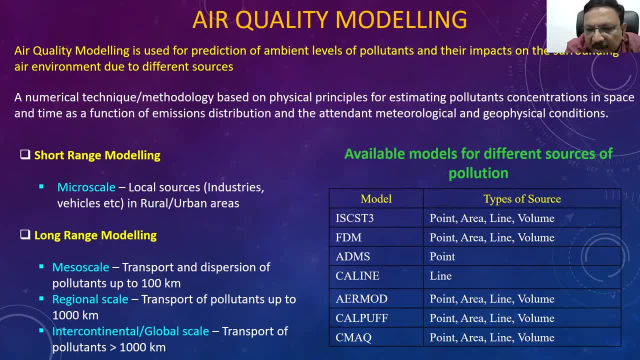 And the area of dispersion And the area sources wherein landfill sites, municipal solid waste burning, domestic waste burning, mining related or dust excavations, construction activities, all those can be considered as area sources. And the line sources are the automobile sources playing on the roads. 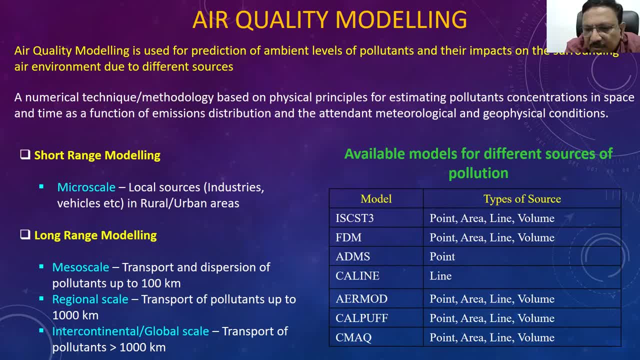 The emissions from the vehicles can be taken as line sources and volume sources. Different types of the models are available for use in the microscale, That is, in the urban scale. That is in the urban scale. That is in the urban scale. 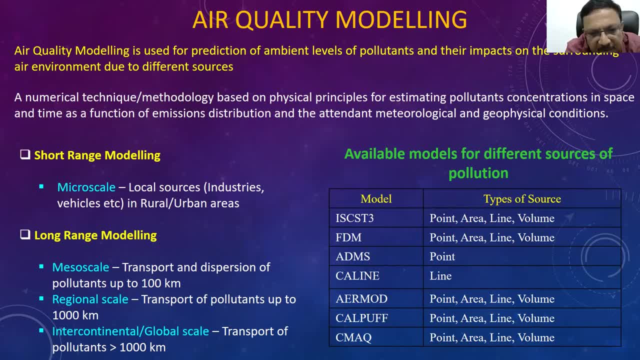 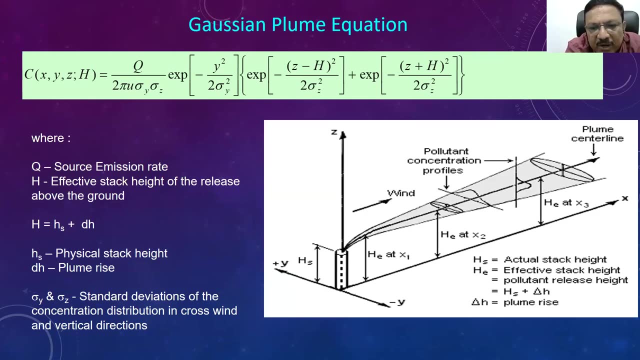 That is, for local sources wherein different types of sources like industries, vehicles and other activities taking place. And next slide, please. All these models, basically in the microscale, are a solution to adversion diffusion equation wherein the normal distribution is considered an equation for elevated point sources, for 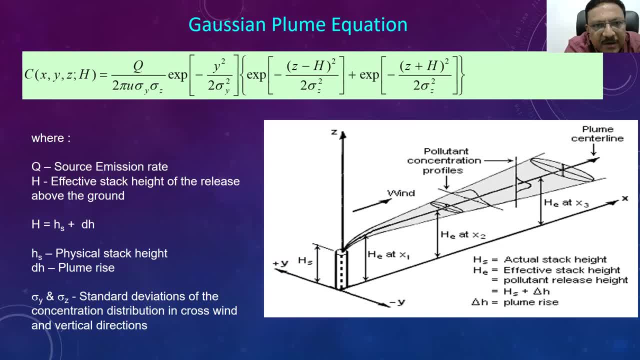 continuous emission of sources Can be written. And then the next slide. This is very easy to understand And can be written. An analytic equation can be in the form of Gaussian-Provitz equation, wherein the concentration is cubed upon exponential minus. 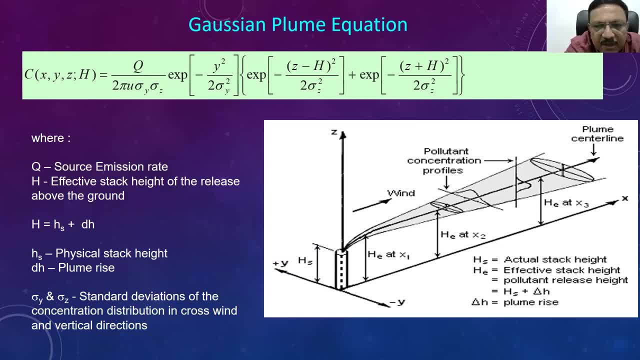 Exponential term in the vertical also will be there, And the figure…. If you see, elevated sources is nothing but a stack coming out of which is moving along the X-axis direction, and the wind is taken along the X-axis direction. like that and with 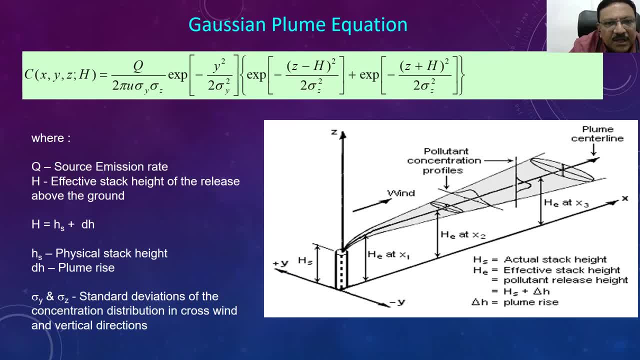 some assumptions, the equation can be brought to the Gaussian plume equation, wherein we need to have the information in the Q: the source emission rate, that is, the pollutant released per unit time In the plume rise. the effective stack height will. 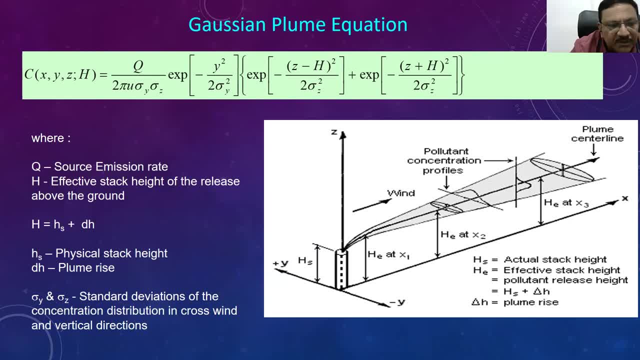 be the summation of the physical stack height and the plume rise and the standard deviations of the constant distribution in the crosswind and vertical wind directions, which are available from the integrations and tables from the literature can be used and we can get the 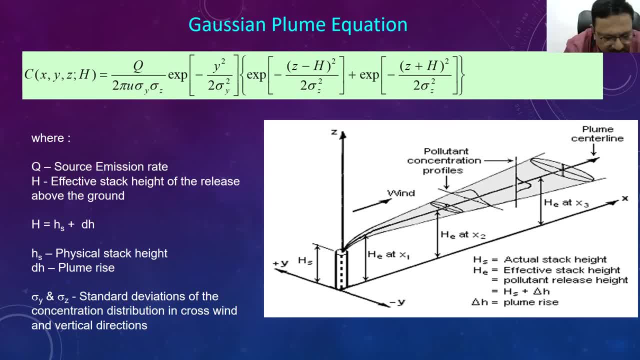 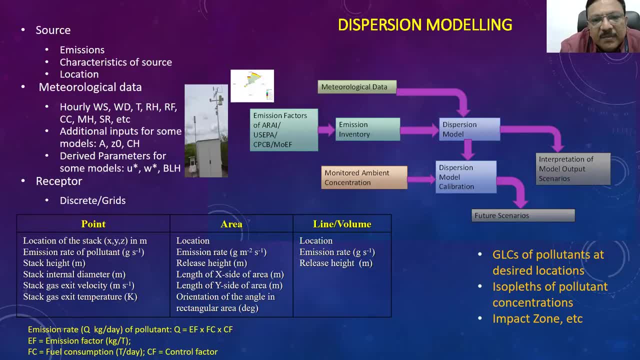 concentration at any desired location in the horizontal and vertical levels at any given point of time. Next slide, please. So basically, many models which we have seen in previously will be using that, using this equation. basically, The dispersion modeling is primarily having modules like emission inventory. that is nothing but the 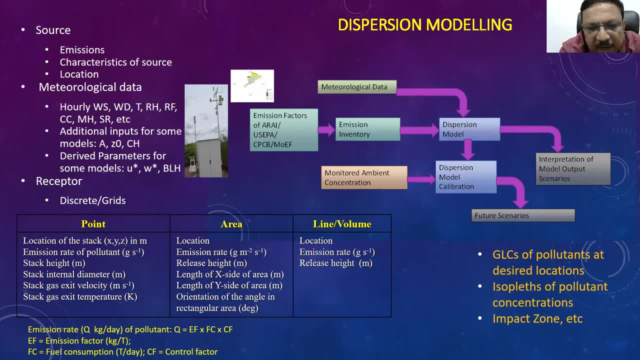 information on the source- polluting source, like the height of the stack and its characteristics, along with the pollutant emission rate- how much it is getting emitted per unit time, and meteorological data and monitored ambient air quality concentrations. All these will be given as input to the dispersion model. 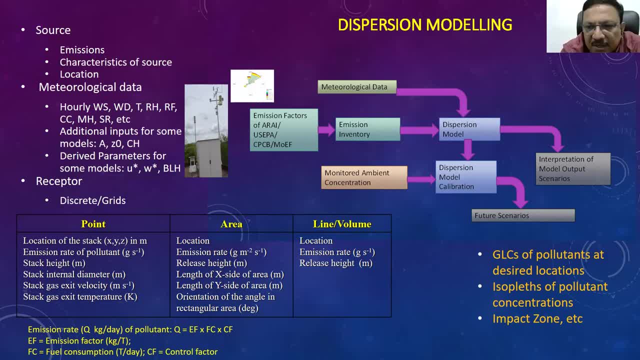 and the dispersion model will be calibrated using the monitored ambient air concentrations, Like in the previous scenario. in the previous lecture paper. Padurama, madam, she talked about the business-as-usual scenario and the projected scenarios wherein we can have the information on. 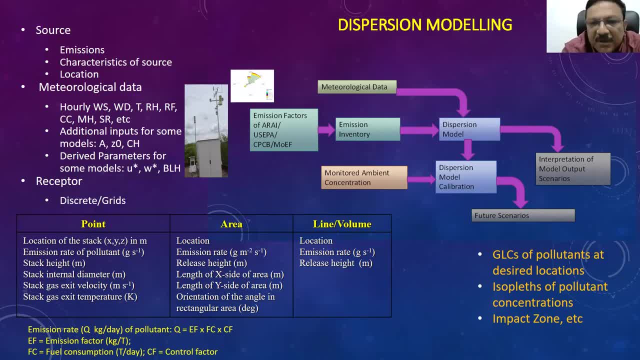 the emission inventory, the hotspots of emissions in ICT can be identified and we can use those information in the graded form- Next slide, please- And across the city, from the hotspots how they are getting dispersed and how they are impacted in the entire city in the form ofISOP nets we can have. 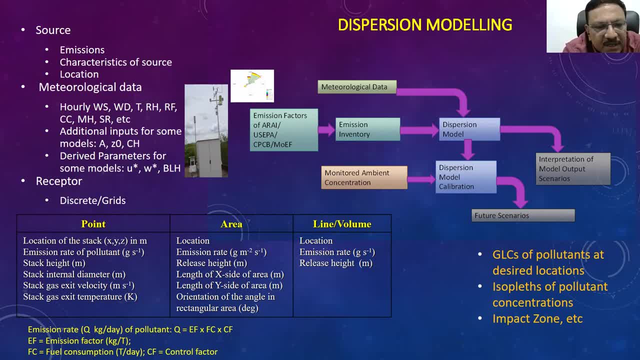 information on that. As I said, the models require the information on the source, that is, emissions at their location, and the setting point that is elevated to stack location of the stack emissivity of the pollutant in grams per second. ждelt for fries quality, creatinine, etc. to 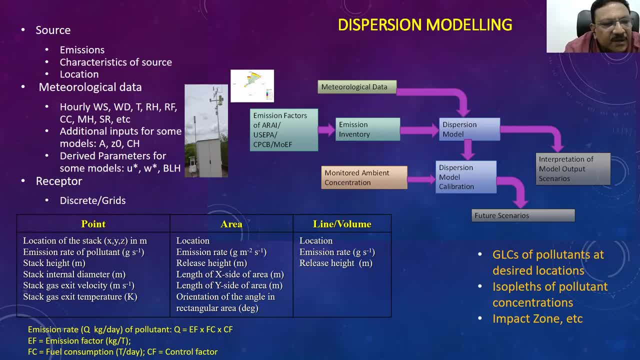 told them how it is getting enrolled and how this might increase. Now it is possible to emission rate of the pollutant in grams per second. stack height, stack internal diameter, stack gas exit velocity and exit temperature And along with it. 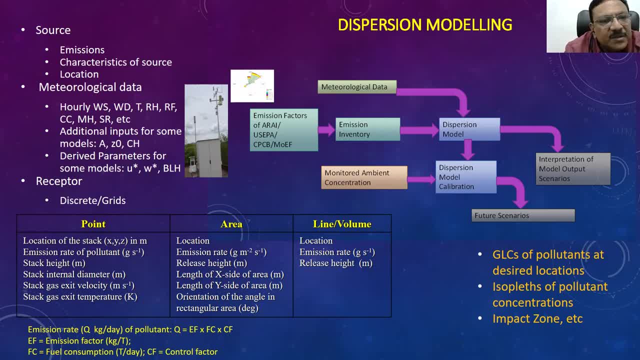 we need to have the information on the meteorology at hourly: wind speed, wind direction, temperature, relative humidity, cloud cover, mixing height, solar radiation, etc. And albedo and ceiling height and the surface roughness length to know the surface friction velocity, U star and convective velocity scale, W star, mixing height. All these can be derived using some meteorological models as well or using the implications one can have it. 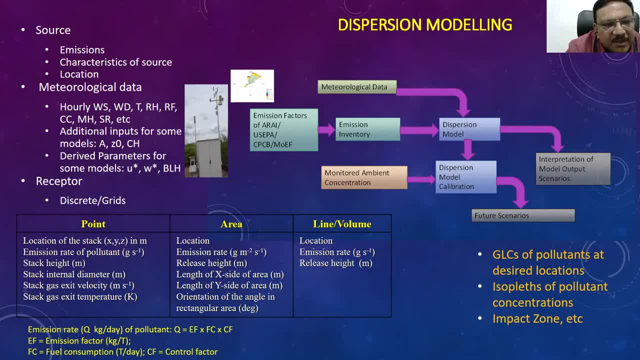 And the concentrations can be obtained at a given receptor, like any discrete receptor wherein we can estimate, or the entire city, when the graded emission inventory is there. because of those emissions across the city we can have several grids and in each grid point we can have and we know the distribution of the pollutant concentrations over there. 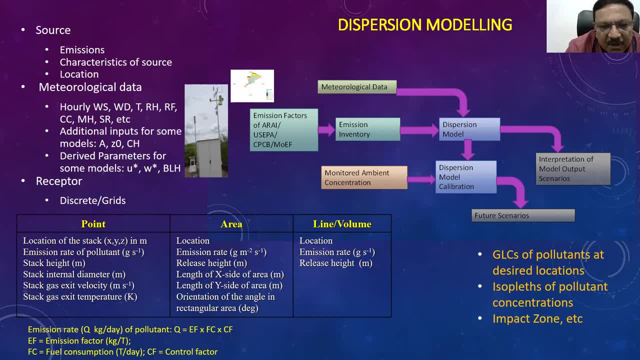 And based on that we can have city action plan also can be improved or generated like that And similarly, apart from the point sources, we have the area sources for which the location emission rate in grams per second per unit area is required. release height from which? 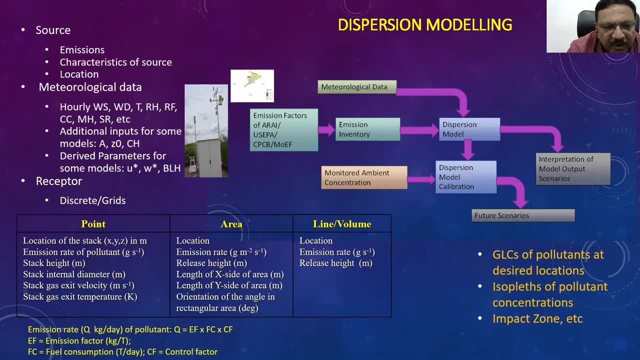 height the emission pollutants are being emitted and length and breadth of the area source and orientation of orientation angle of the rectangular area or the area source with respect to the north is given, And similarly the linear volume sources. the location of the source, its emission rate and release height is required wherein the regular sources are treated. 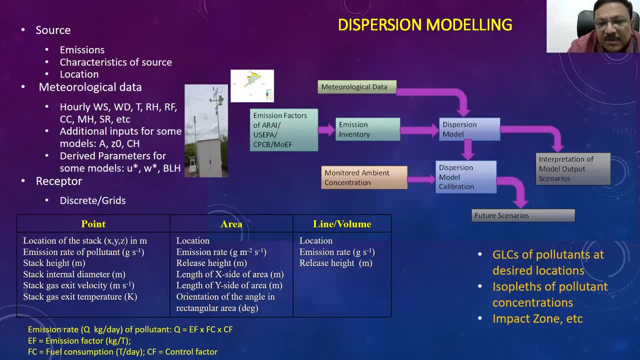 as a single point. the entire road on which the vehicles are playing will be treated as an individual point points or a small, infinitesimal small point sources and integrated along the road to get the concentrations. So the dispersion model can. 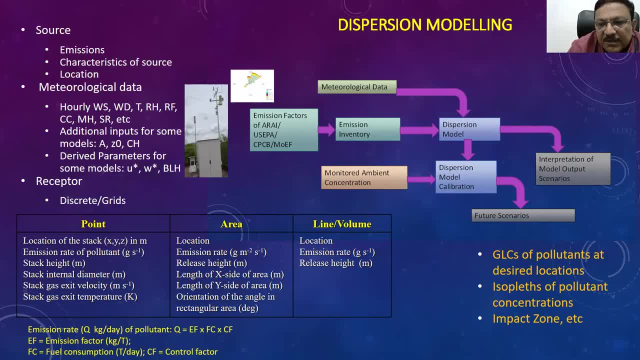 be utilized for getting the pollutant concentrations, to know the level of pollutants individually and to calculate the air quality index of that city or urban area and to reduce that. what are the action plans required to reduce the emissions at the source or after coming into the atmosphere released? once released into the atmosphere, how it can be curtailed like? 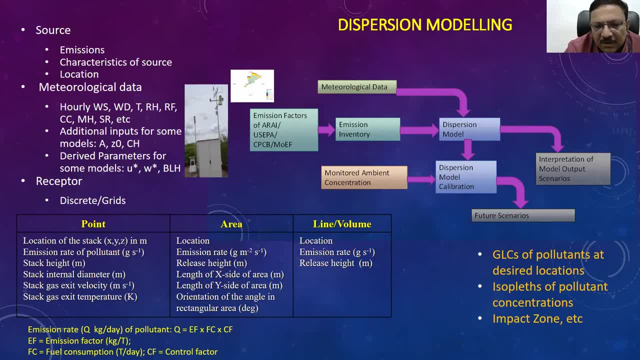 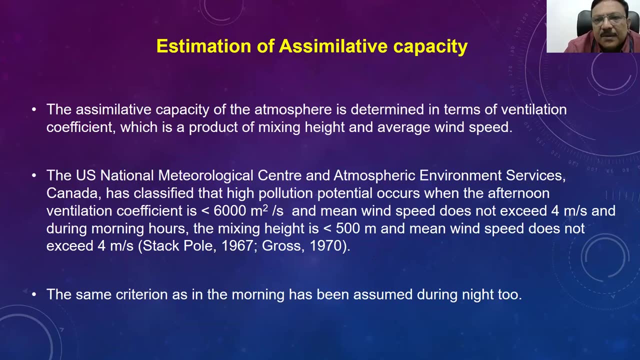 using various smoke towers like that to reduce it can be considered to, so that the levels of pollutants can be brought down, brought down to the better air quality index levels. Next slide, please. And this is: the espionage capacity is a kind of calculation, which is which gives information about defining a deletion of an airshed. 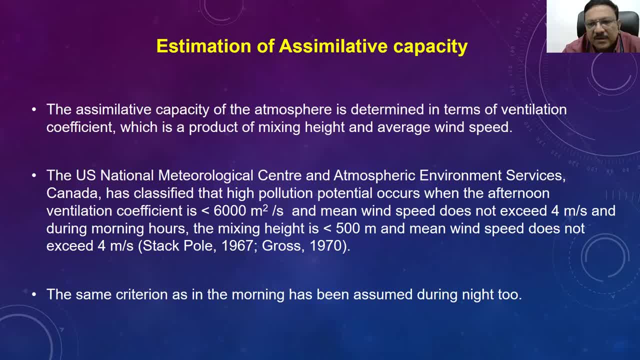 If any, any city area wherein we have information on the mixing height and the average wind speed of that area. the product of the mixing height and the average wind speed will give us the ventilation quotient. So the espionage capacity of the atmosphere can be determined in terms of ventilation quotient, which is a product of mixing height and the average wind speed. 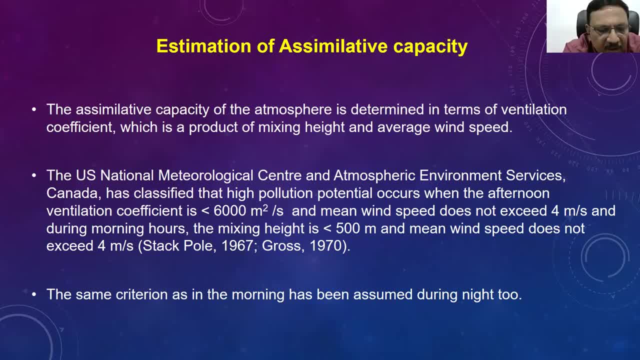 The US National Meteorological Center and Atmospheric Environmental Canada has classified that high pollution potential occurs when the afternoon ventilation quotient is less than 6000 meters per second and wind speed does not exceed 4 meters per second. during the morning hours, The mixing height is less than 500 meters per second. 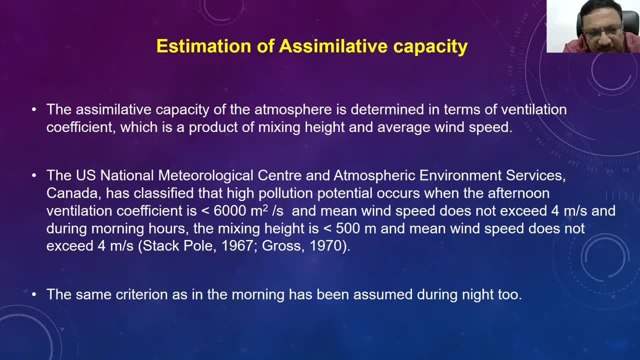 And the main wind speed does not exceed 4 meters per second, A criteria given by the Stackpole and Cross back in the 70s, which can be still utilized. as for estimation of the espionage capacity of that region, up to what level, up to what extent can be the pollution can be taken? 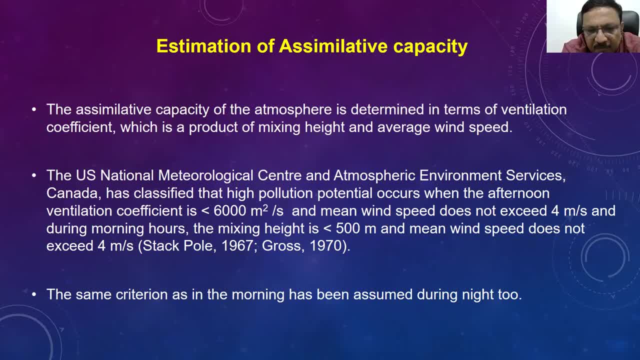 by those cities because of various different sources. So the same criteria of morning hours can be assumed during the night time also, And I would like to. having discussed about the dispersion modeling and the espionage capacity definition, I would like to share some details on the. 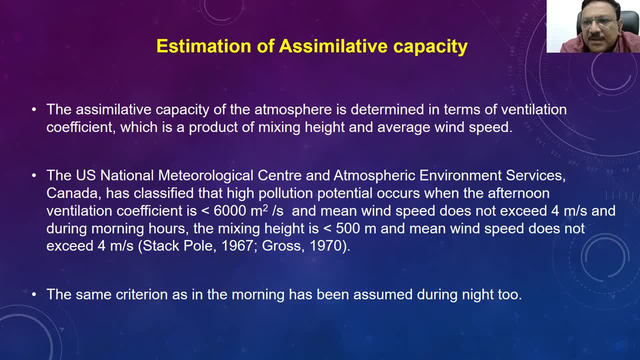 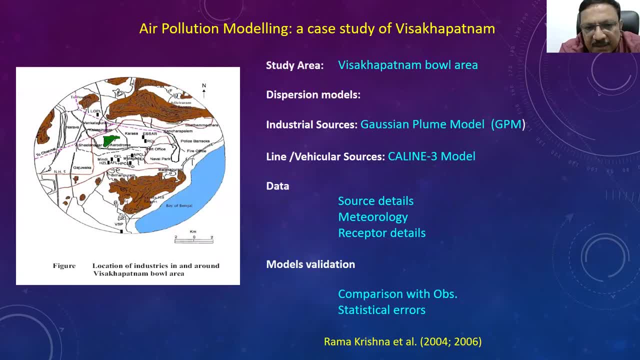 case studies wherein we have studied the dispersion of the air pollutants. Next slide, please. Next slide. By application of different models, we can know the dispersion of air pollution over a city and urban area. In this case, for example, we have taken the Vishabhutin-Bohal area as a study area. 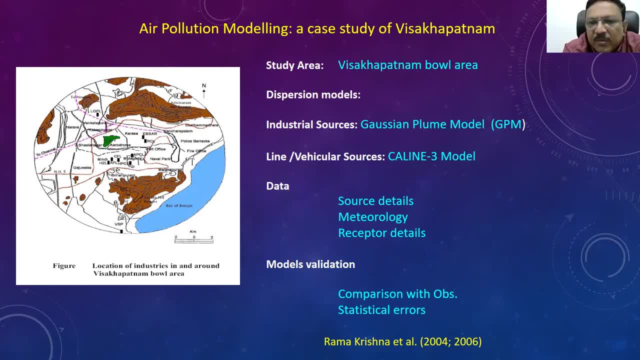 wherein we have taken the major industries of about 9 to 10 major industries, of which 67 stacks- existing stacks were considered- And the industry sources. the stack details and emission rates from these stacks are used as input to the Gaussian Probe model, which was discussed earlier. 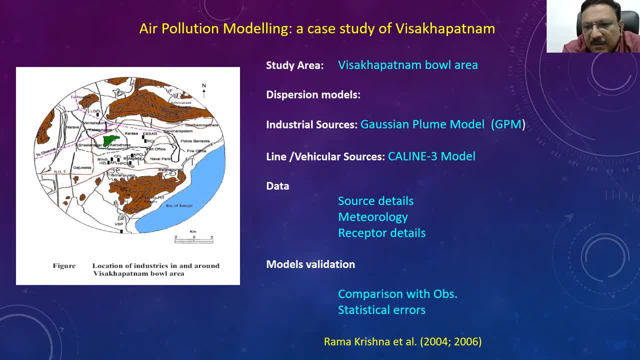 And the vehicular count data taken and we have calculated, estimated the emission rates of the pollutants from the vehicular data and road length data And the Callahan 3 model is used for estimating the pollutant concentrations due to the line sources And the data, as I said in the previous slides. 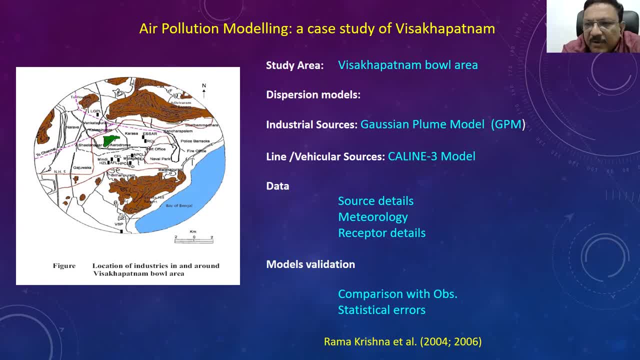 the source details, the metallurgy, the hourly wind speed, wind duration, temperature, relative humidity, cloud, core assets, solar radiation are being given And we have taken discrete receptors at desired locations, at locations where the ambient air quality was monitored, so that we can compare with the 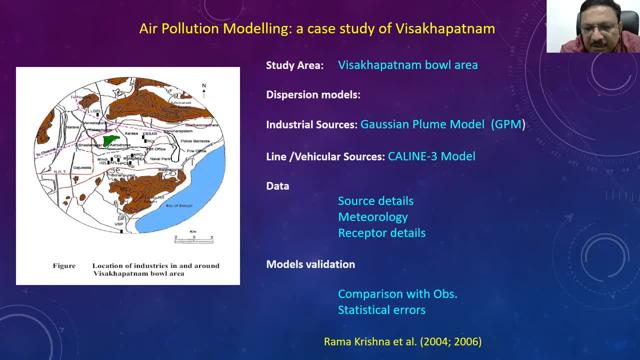 observed data And the model. validation is done by comparing with observations And some statistical errors have been computed. This study has been done for the Vishabhatnam Bowl area way long back. The next slide will give us the definition of the ventilation quotient. 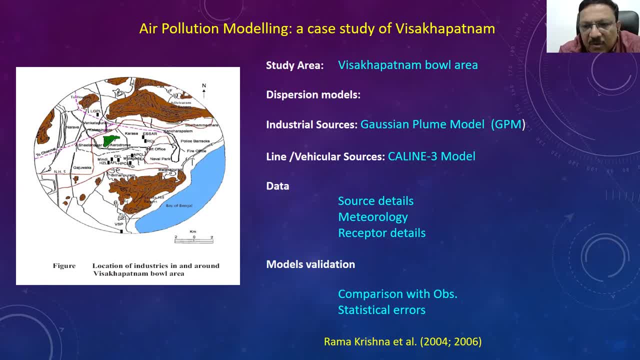 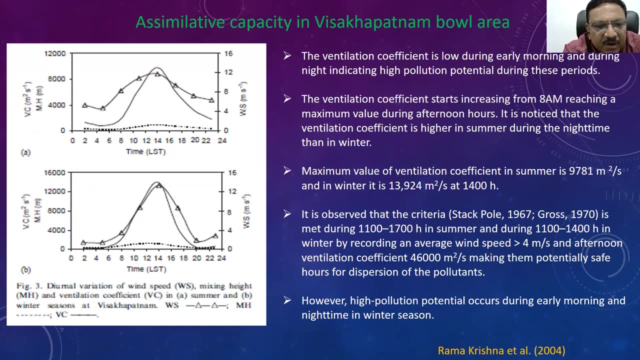 wherein the similarity capacity of the Vishabhatnam Bowl area using the mixing height and wind speed data we have estimated. Next slide, please. We have estimated the ventilation quotient And in two different seasons, summer and winter, wherein hourly mean wind speeds at the mixing heights were taken. 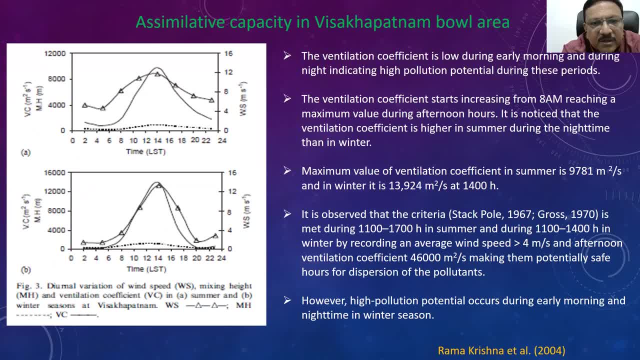 and the product of which both will give the ventilation quotient in meter square per second. The ventilation quotient observations are like this: It is allowed during the early morning hours and during night, indicating high pollution potential occurs Because the stack-pole criteria tells us that less than 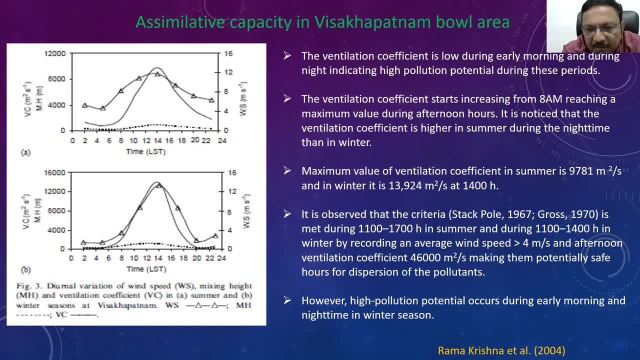 6,000 meters per meter square per second, and the main wind speed should not exceed 4 meters per second, The pollution potential will be high. Here. the pollution potential is observed during 11 to 17 hours. That is the daytime. 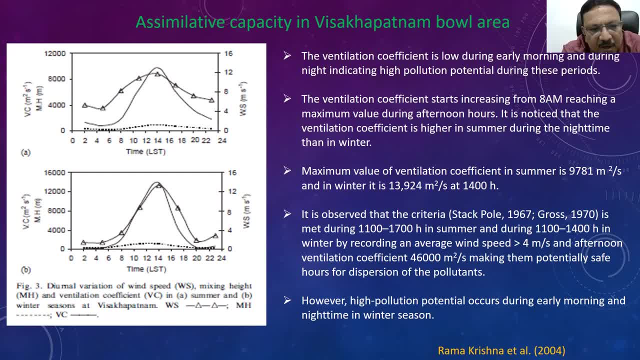 In both seasons we have low pollution potential. That means it has higher vicinity capacity, wherein the pollutants can be safely released in those hours. However, in the early morning hours and in the late night hours the high pollution potential will be high because of the lower vicinity capacity. 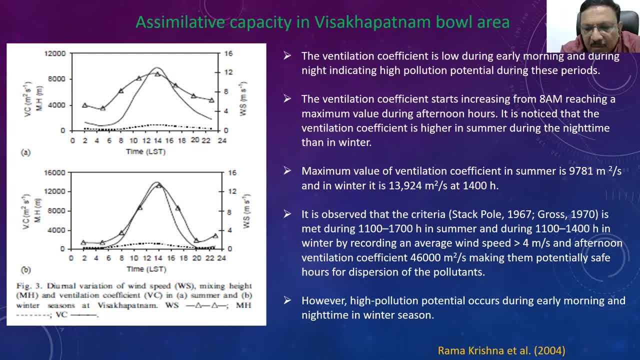 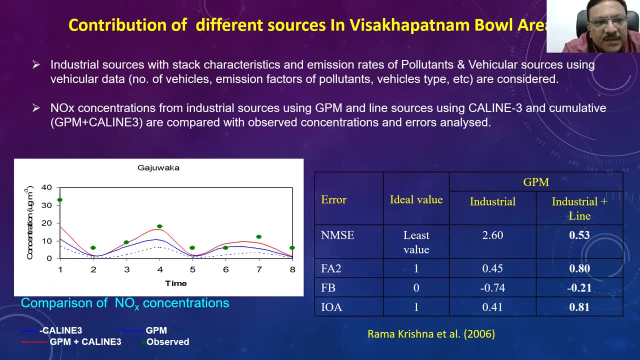 or the values of the ventilation quotients are not meeting the safe criteria of the pollution potential. Yeah, then next slide, please. And here, as I said before, in the Vishabhattinbohar area we have industrial sources for 9 to 10 major industries. 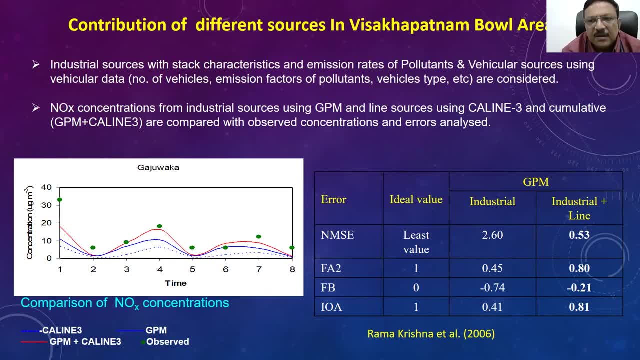 with 67 stacks. data is given as industrial source And the regular data at different traffic intersections were counted and the emissions were calculated based on the emission factors of the pollutants and for different vehicles types and the road length, And using the these two we have used the Gaussian proof model. 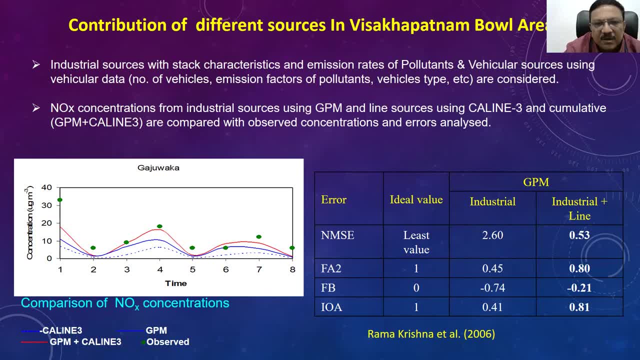 for industrial sources alone and Kalain 3 model for vehicle sources alone, And then we combined together to combine together to compare with the actual model values at those ambient levels of pollution, set one particular station here And this is just a representation purpose. That's what I have given it. 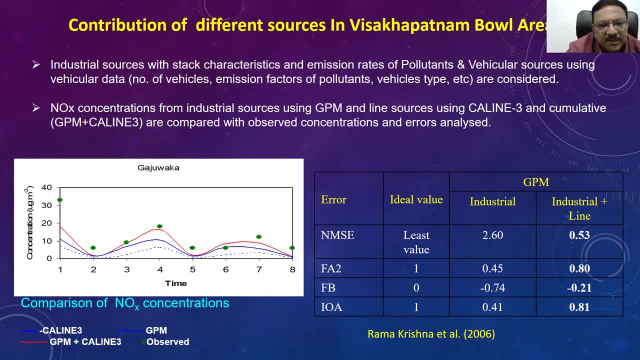 If you look at it, the blue- solid blue line gives the industrial sources alone data estimated values and the dashed line gives the Kalain 3 model results. But when we combine both, so when we can consider both the sources, and they're very well in agreement with absolute values. 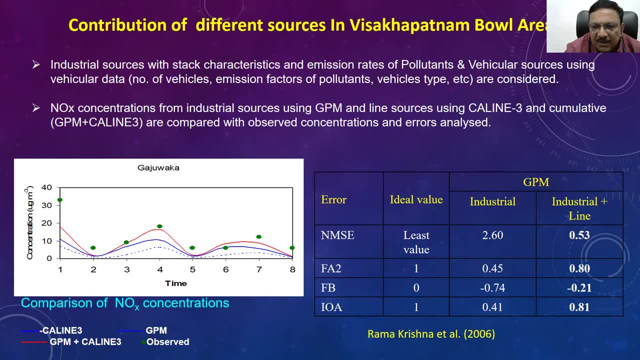 And similarly these concentrations were subject to the sub-statistical analysis, normal scale error, Fraction of rational bias, and this equipment like that, And we have found, when all the sources considered, using different models, or even nowadays here, what can treat all the types of vehicles, like the calc, of all type of sources you can have. 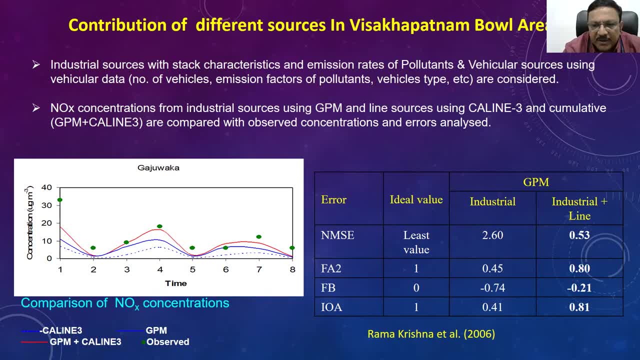 and the pollution concentrations can be estimated Like this: the concentration of all these sources is required to get the exact representation of the pollutant levels in that particular area. And the urban areas are cities which we are considering Next slide, please. 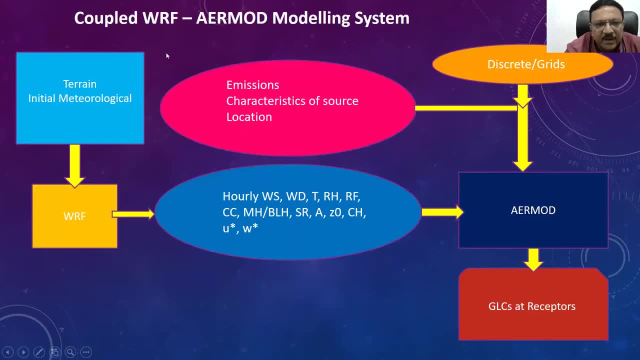 And recently again, a few years back again, we released it by giving more meteorological information in the study area. The same study area is considered wherein we have used a work model, WRF, to predict the pollutant say, the meteorological. 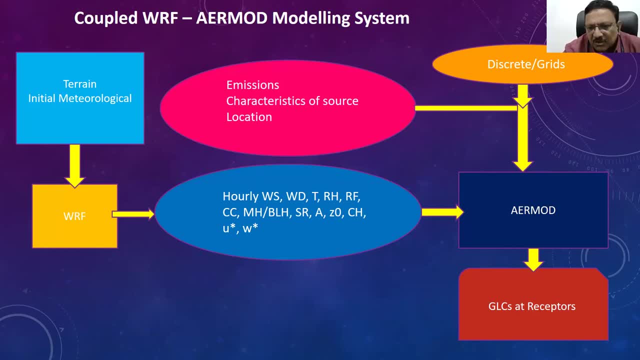 parameters at different grid points. almost three points of meteorological points have come And we combine this with the air model giving the emissions from all the 67 industry stacks and the regular data of the NOx And we calculated the pollutant concentrations. 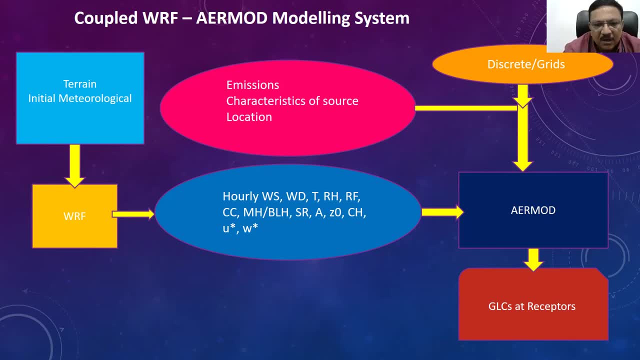 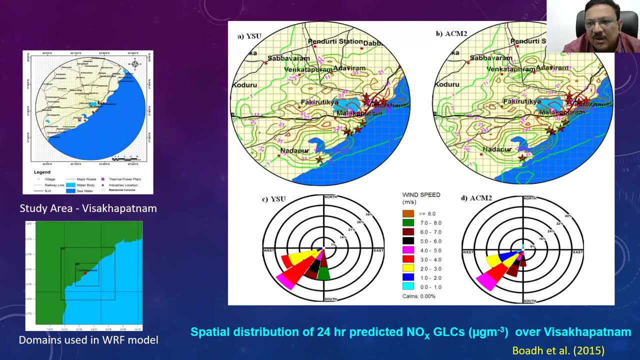 with the combined WRF and air model. And we have seen next slide, please. We have seen the NOx values, because NOx is a major pollutant from the regular sources. We have seen this. This is the same study area we have tested.